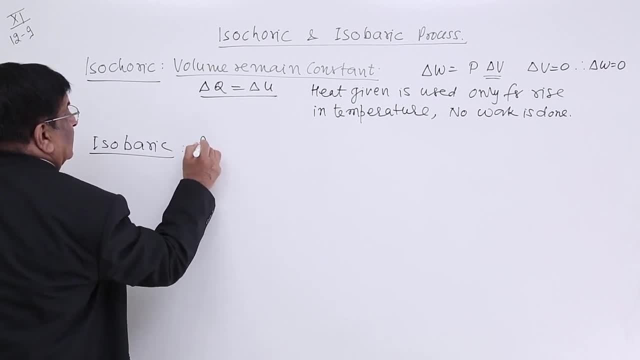 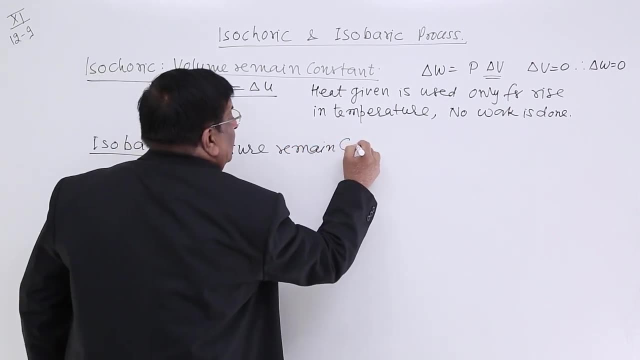 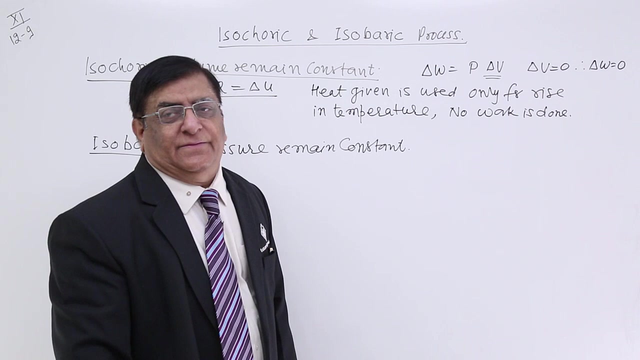 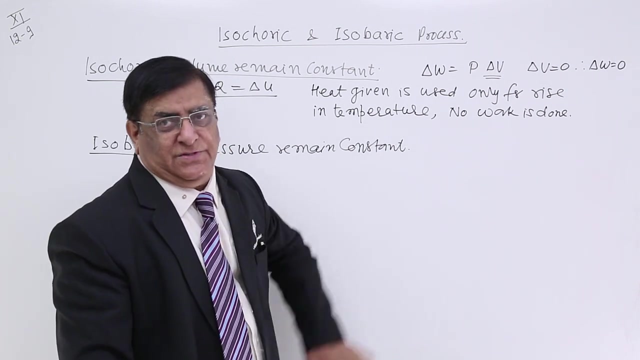 In isobaric process. what remain constant is pressure. pressure remain constant. If pressure remain constant, then how much work will be done? If there is a change in volume allowed, change in temperature allowed, change in heat allowed, the pressure is constant, but work is done. 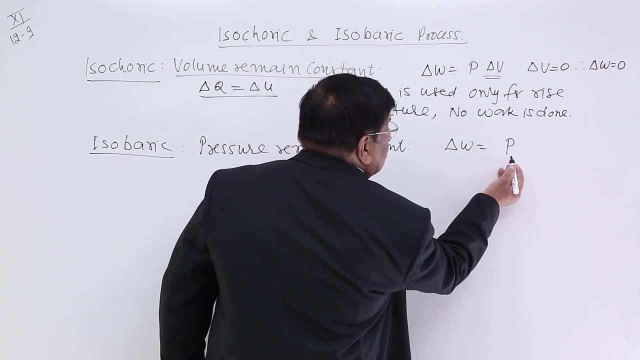 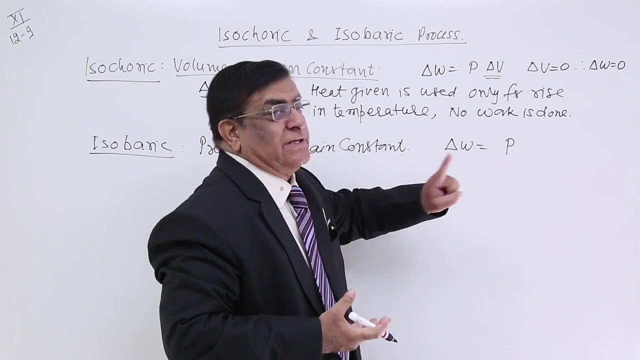 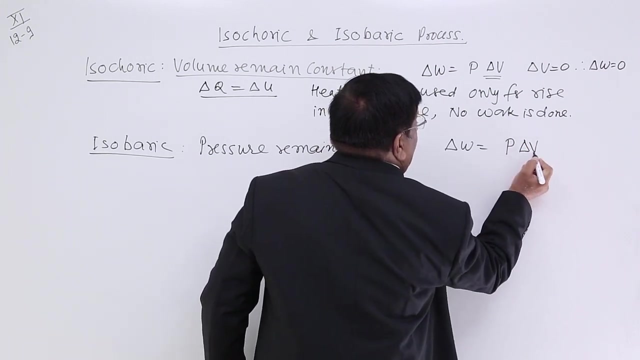 Because delta W is equal to 0. Pressure. this is not change in pressure. this is full pressure and the pressure is there. it is not changing. but we are not using the term delta P, we are using the term only P and delta of V volume is changing. 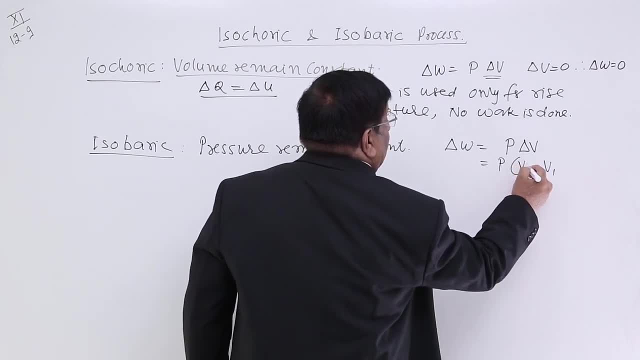 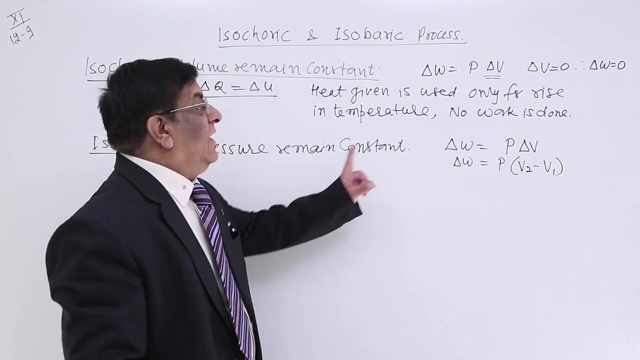 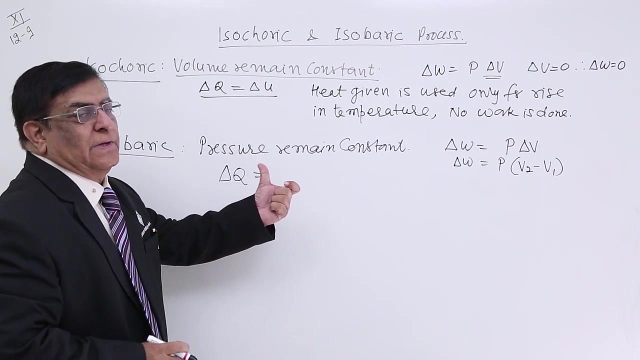 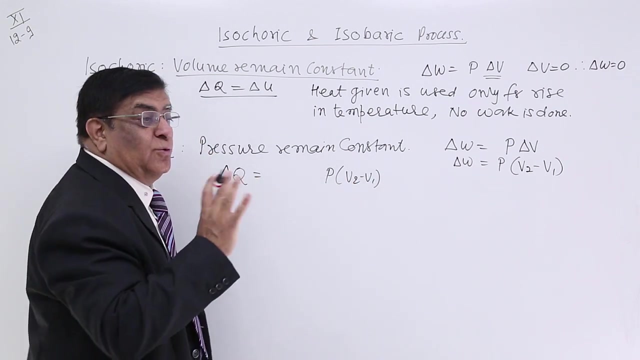 So that is the volume. which was V1 has become V2.. So this is the change in volume. So work is done. of course, Now we are giving heat to the process. Heat, This we are giving to the system. Some work is done, P V2 minus V1, but there is no bar that it cannot take the heat and 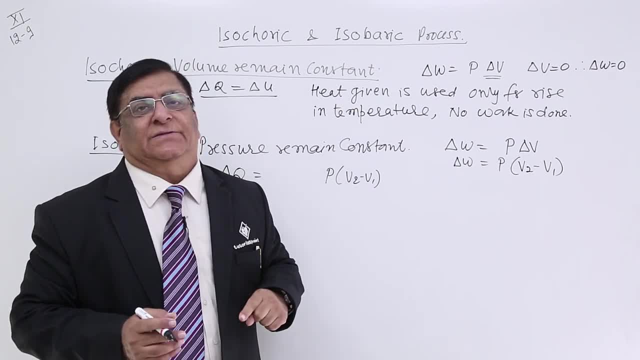 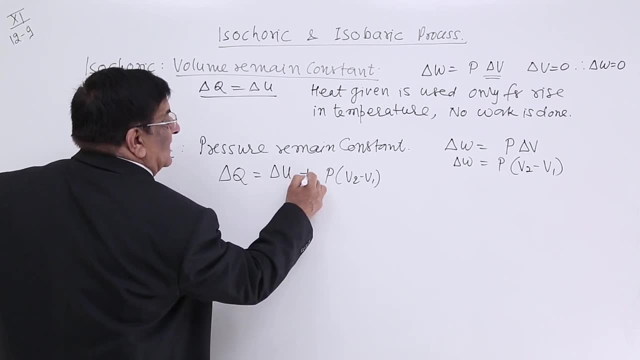 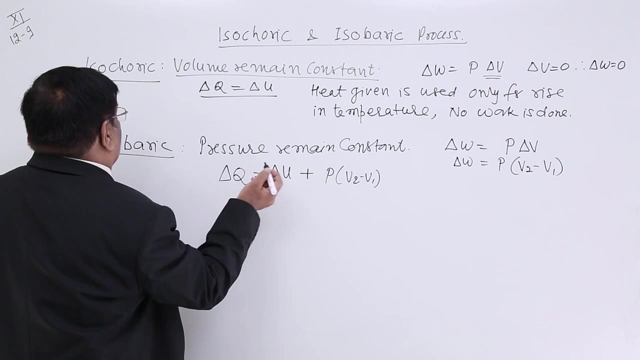 rise its temperature and the system does that. In that case, some of the energy is used for rising its temperature and that energy gives the change in internal energy. So this rise the temperature. So that is what we are giving to the system. So this rise the temperature as well, as work is done. 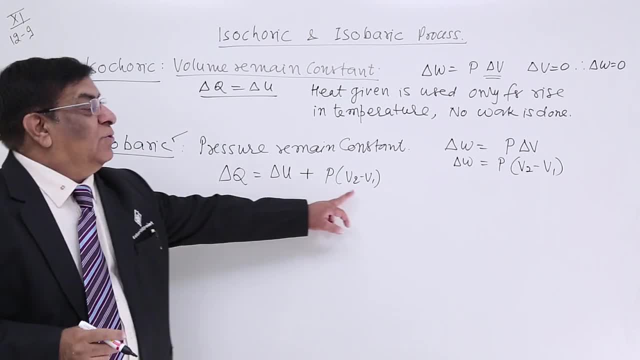 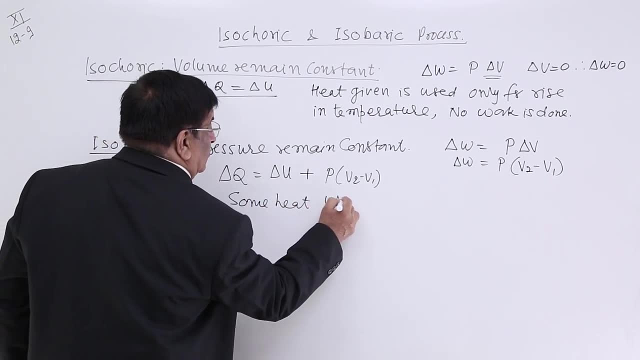 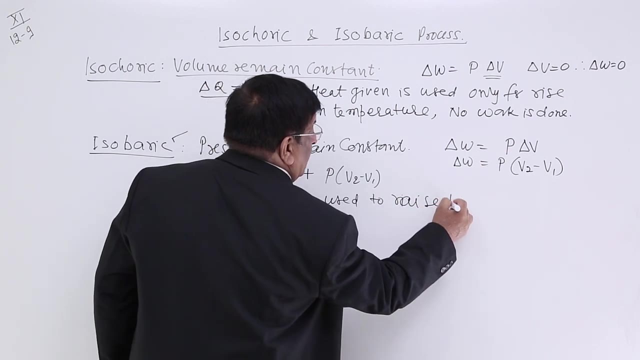 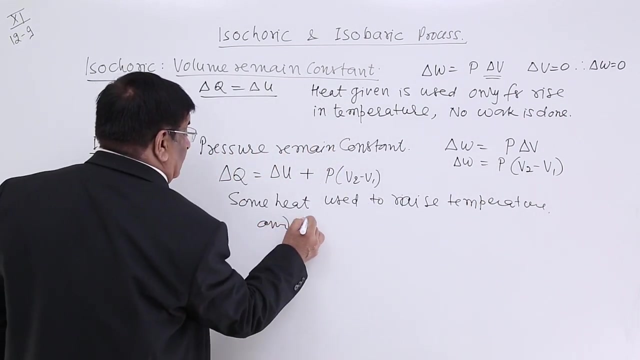 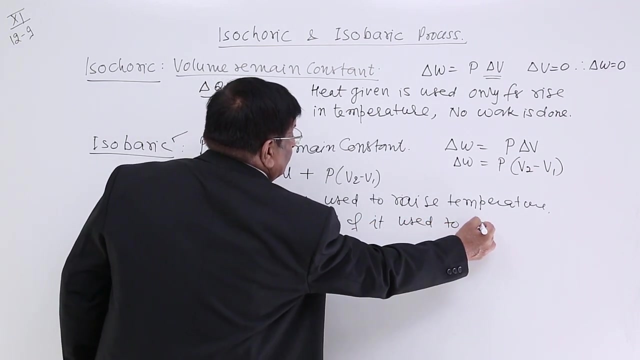 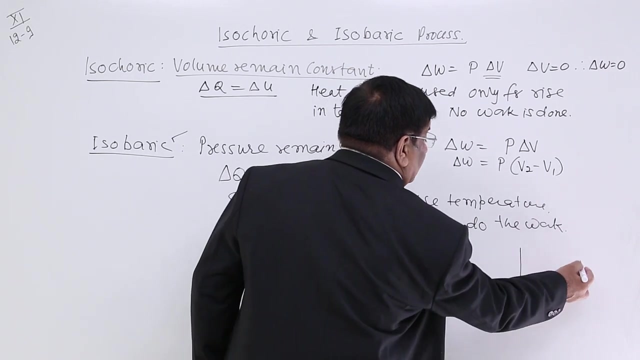 So in isobaric process this whole thing is applicable. Some heat, Some heat used to raise the temperature And part of it. Some heat, Some heat And part of it used to do the work. In a container we take water and heat it. 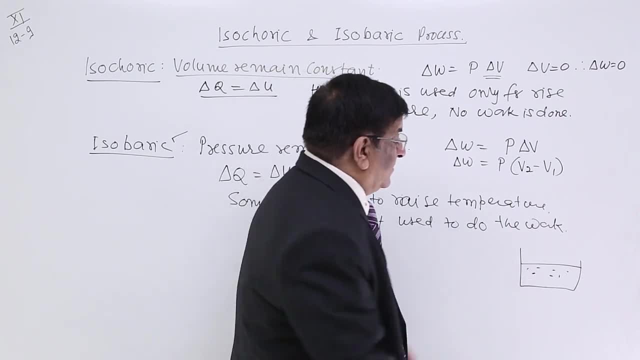 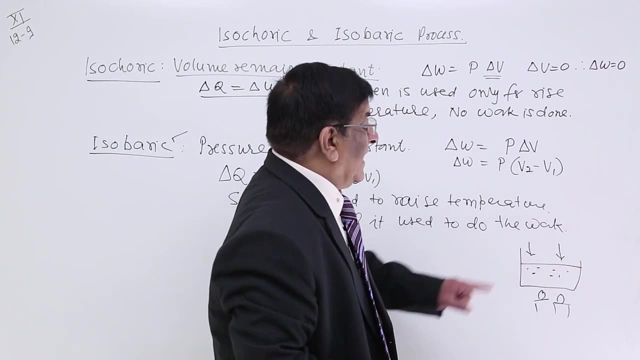 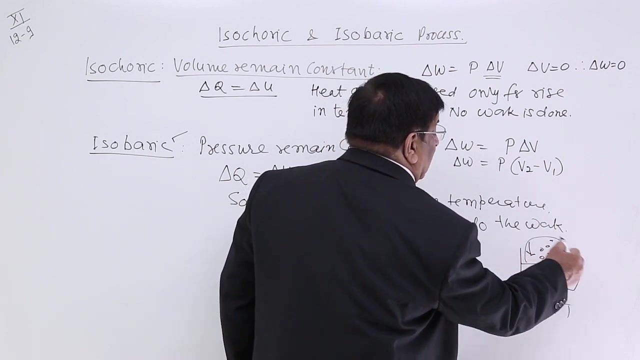 We give heat to it. what happens? There is a pressure on it, Atmospheric pressure. After sometime we find that these molecules are converting into vapor and the vapor starts to form, takes a larger volume. That means there is a change in volume of the system, So converting. 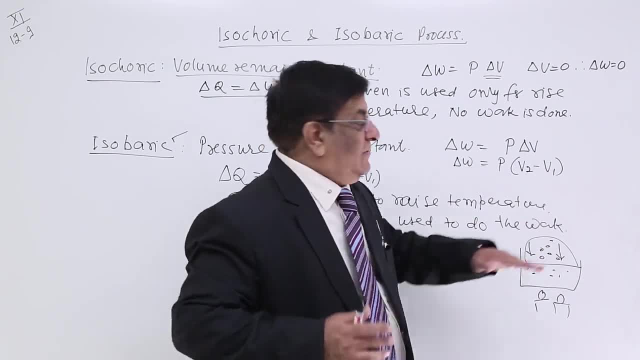 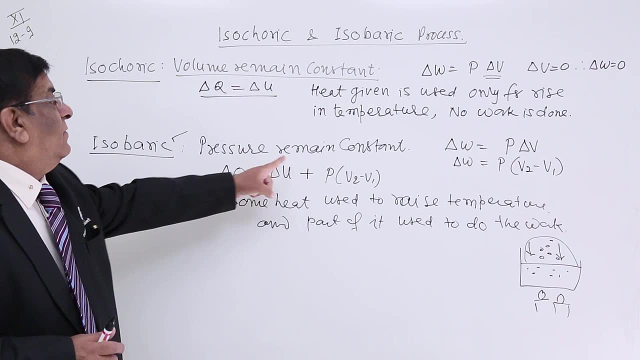 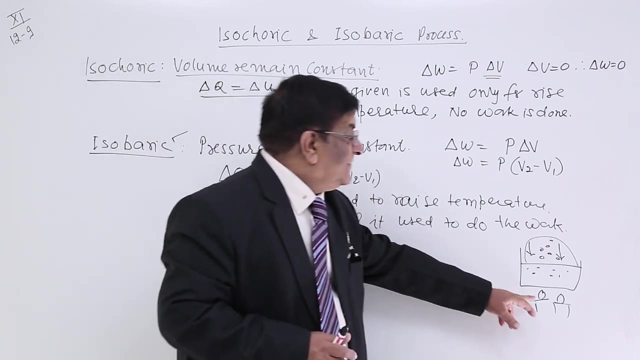 to steam is change in volume, but there is no cap on it. So there is no change in pressure. the pressure remain constant. If the pressure remain constant, what type of process? it is Isobaric. So in this, what happens? The temperature is rising. after this heat, This again gets. 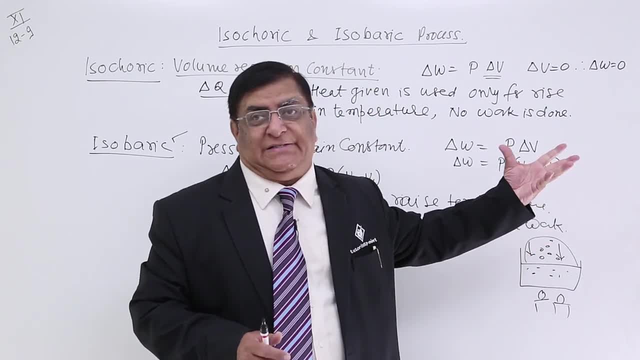 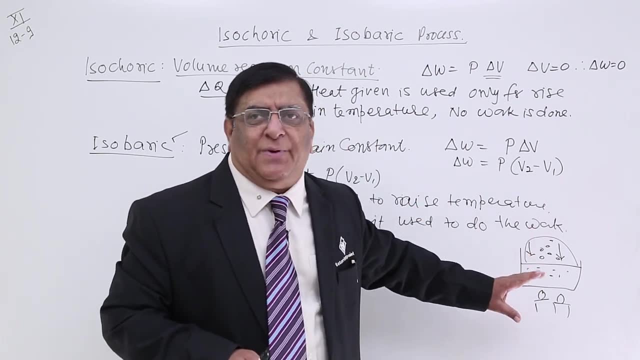 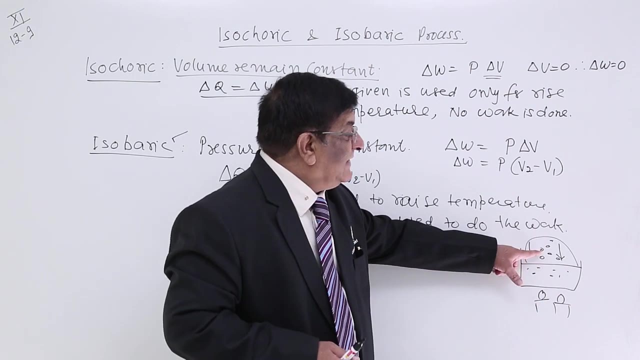 a heat from here and now temperature rise. At the same time work is being done because the volume is increasing. This is one example: The temperature first remain constant At 100 degree. there is conversion. After that, when it gets the heat, it expands, So temperature. 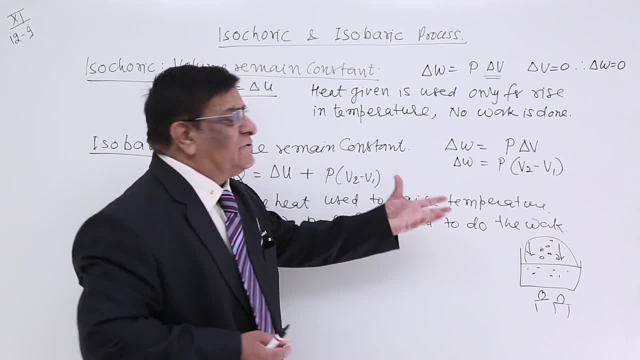 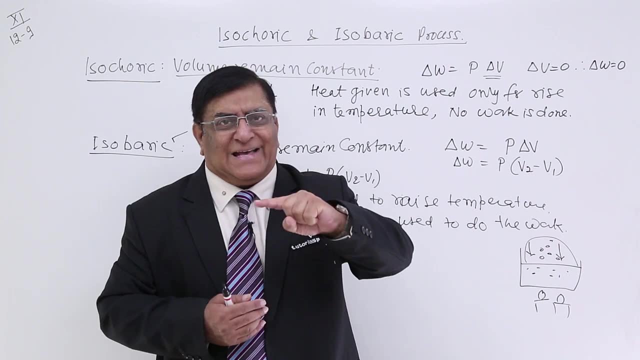 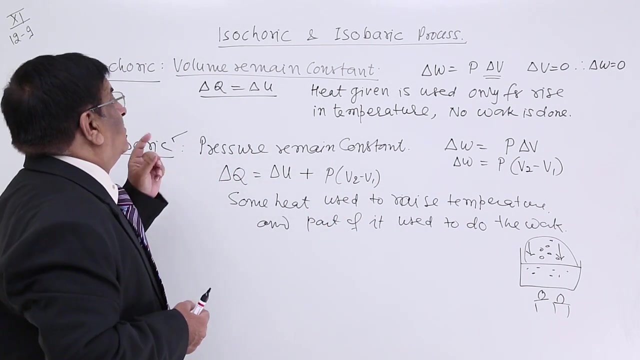 also increase. This is one example. There are many other examples where the pressure pressure remain constant, but the gas gets heated up as well as it expands. that process will be known as isobaric process. this is isochoric, this is isobaric. and there is one. 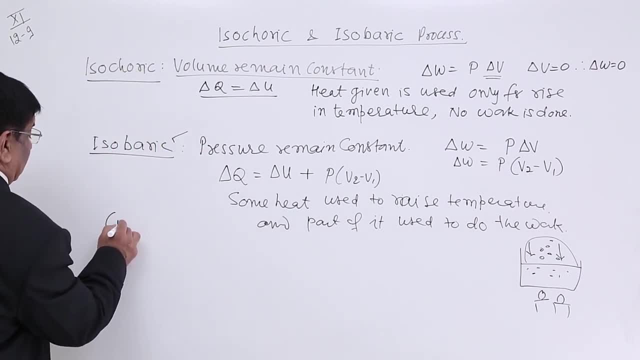 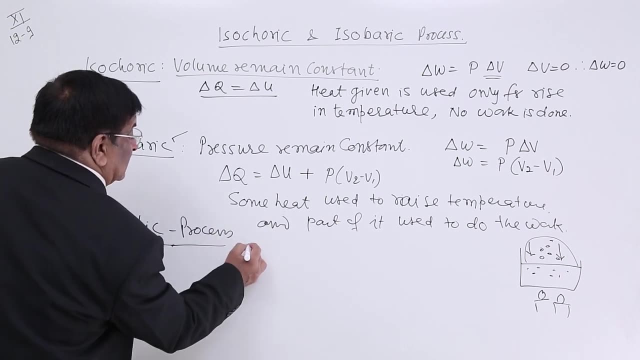 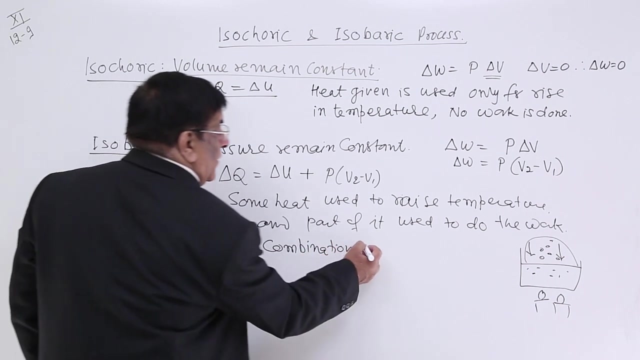 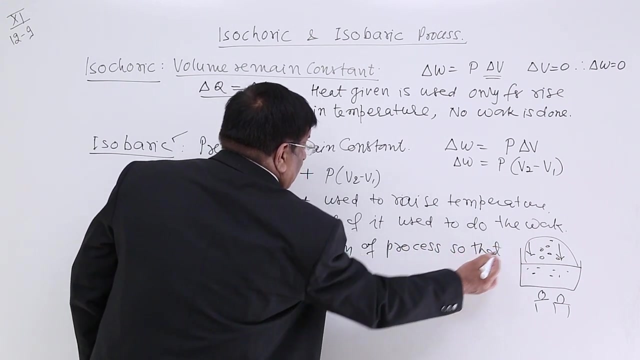 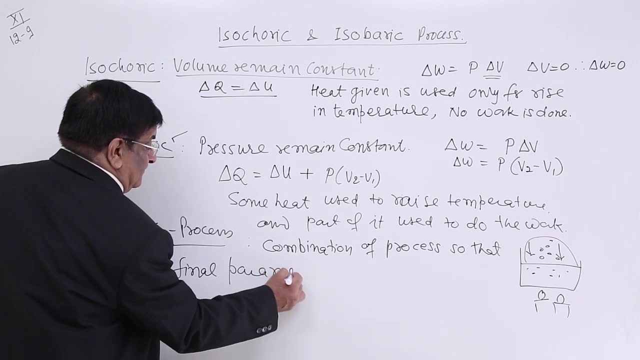 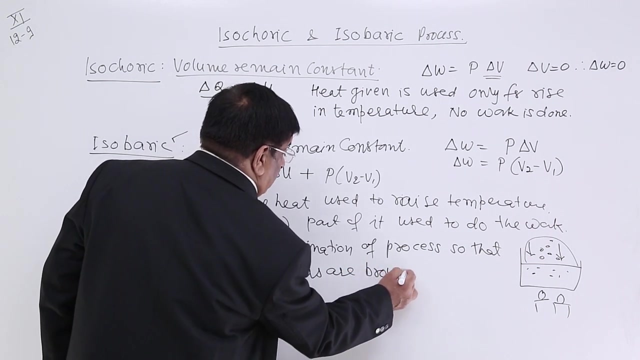 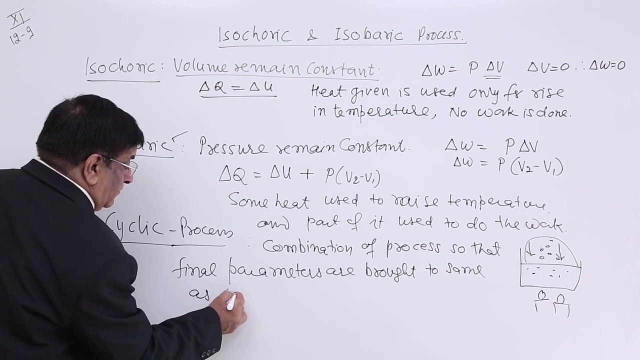 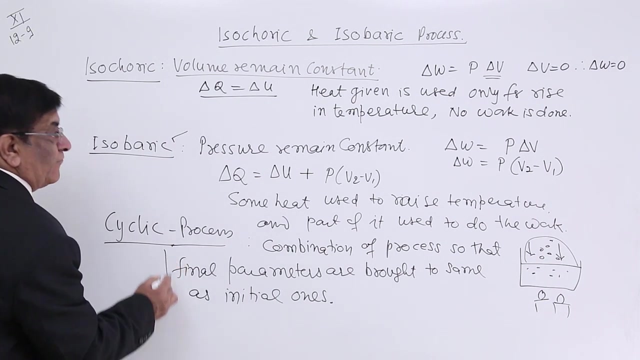 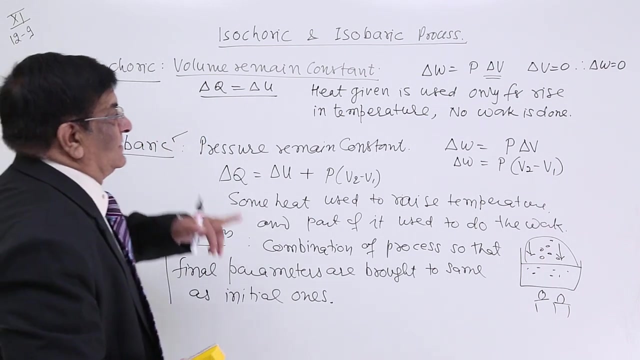 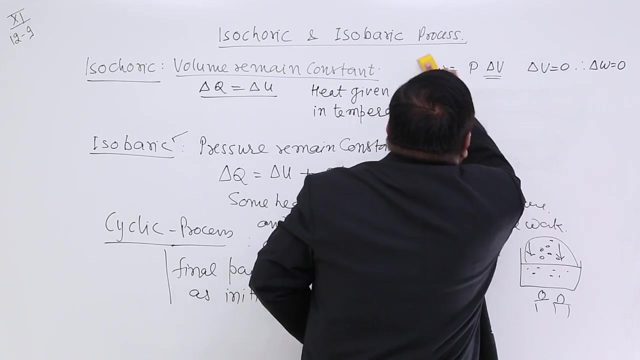 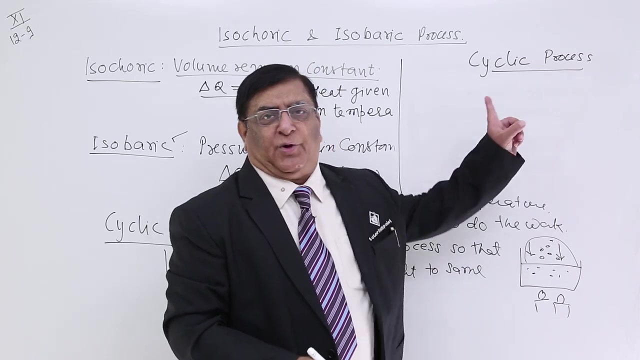 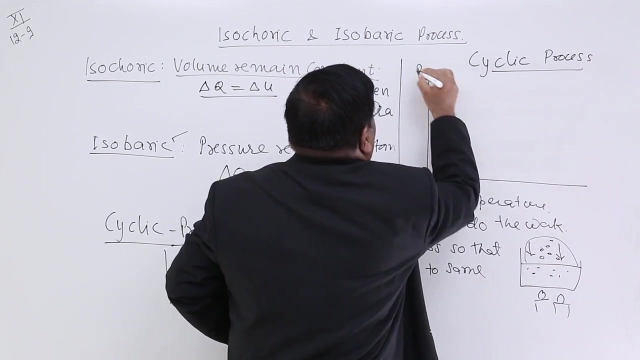 more thing we will study is cyclic process. cyclic cyclic process is not one process, it is a combination of processes so that final parameters are same as initial parameters. this final initial, how can we show it? I will show you here. yes, let me make it here. cyclic process in cyclic process, I make a indicator diagram: PV, at any given time, a. 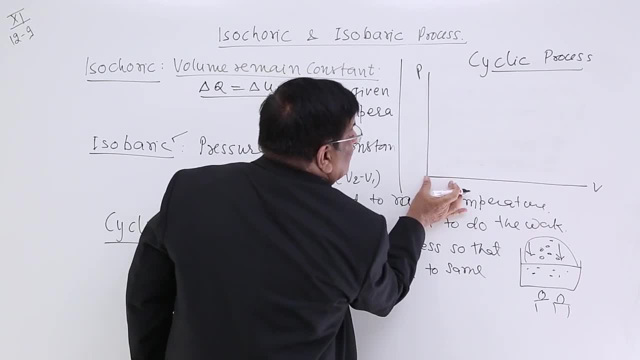 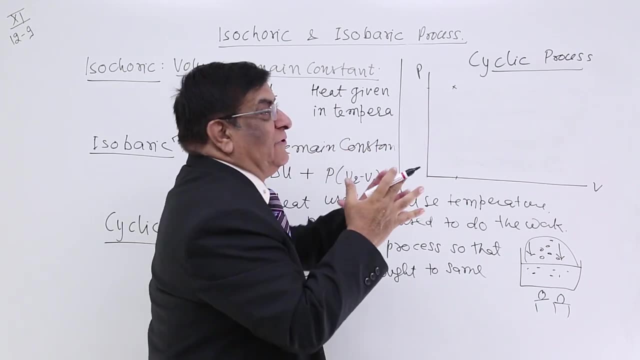 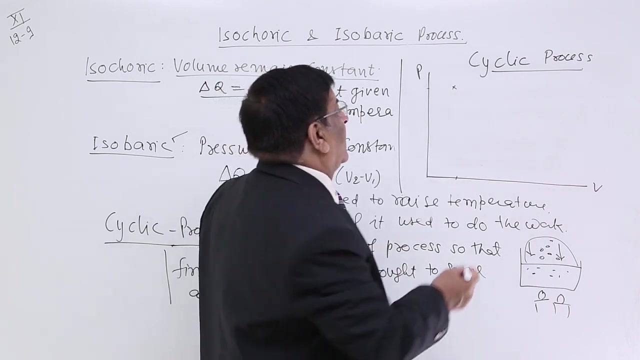 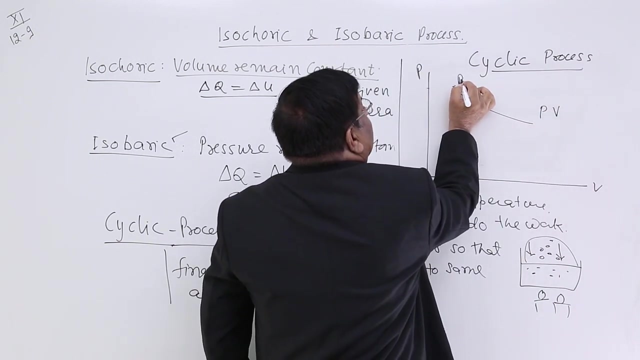 gas has this much of pressure and this much of volume. so this is the starting point: this much pressure and this much volume. after that we do the expansion. suppose isothermal expansion is done, volume will increase, pressure will decrease, will come down and we get a process. Now pressure and volume, both have changed Here. 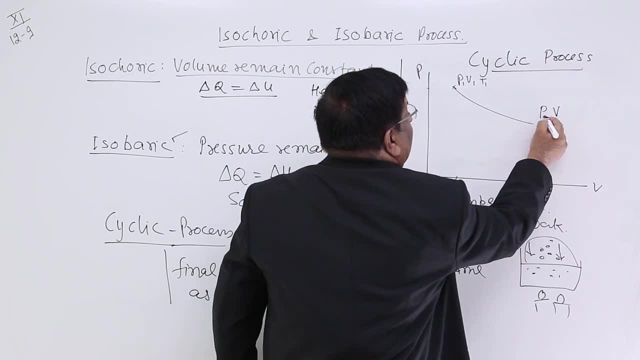 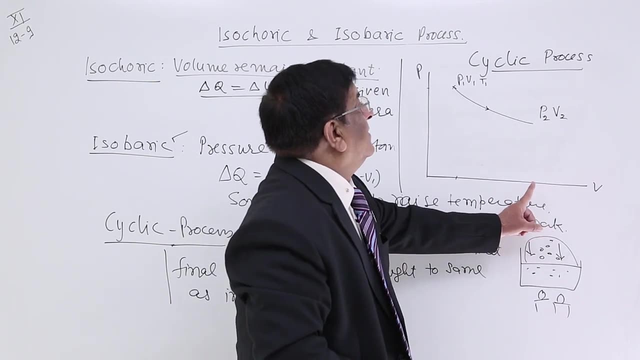 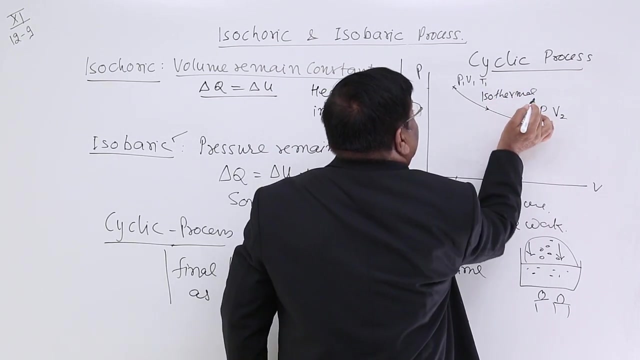 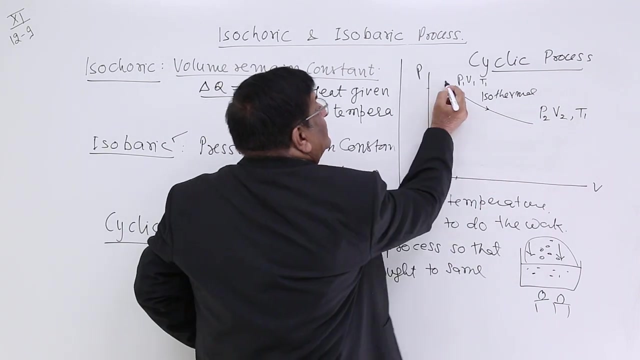 it was P1V1,, temperature was T1, here it is P2V2 and this is an expansion. The volume has increased. This is an isothermal, expansion isothermal, So there will be no change in temperature and I can write here: temperature T1.. After that, we reach this point from A. 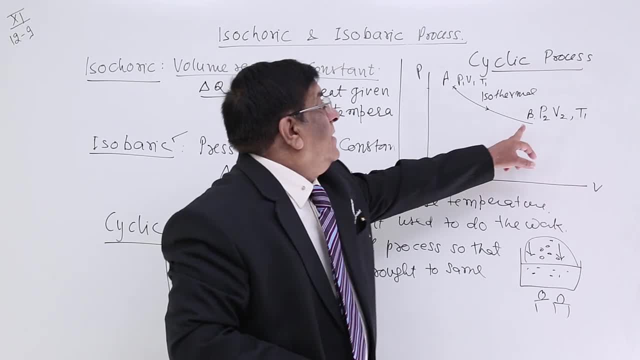 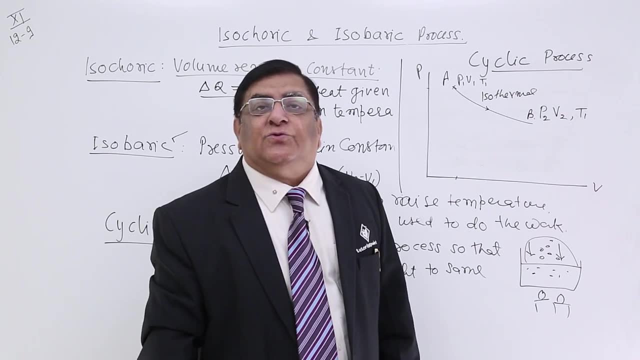 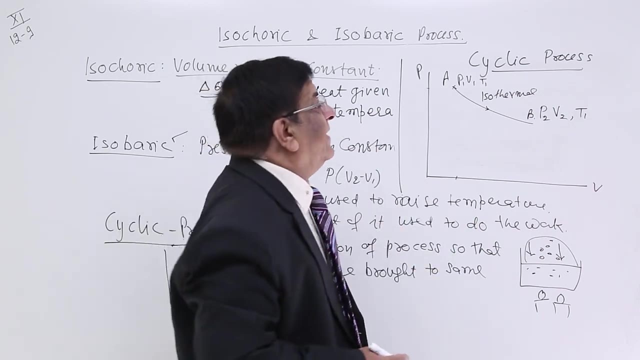 to B. Now at this volume we again expand it, but we do it adiabatically. We do not allow heat to go out, We do it very quick in a insulated pot. Then there is another expansion and with that expansion again the pressure decreases. 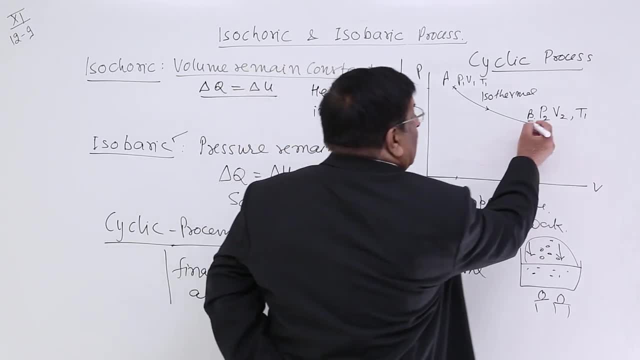 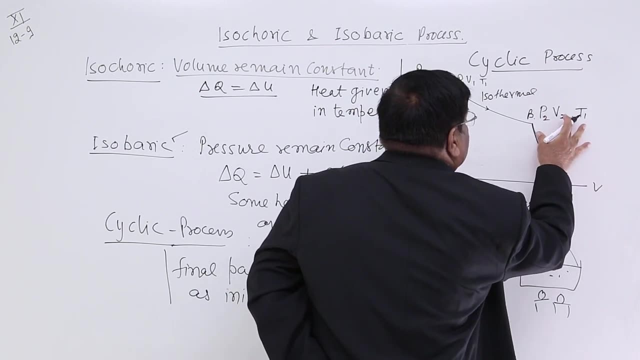 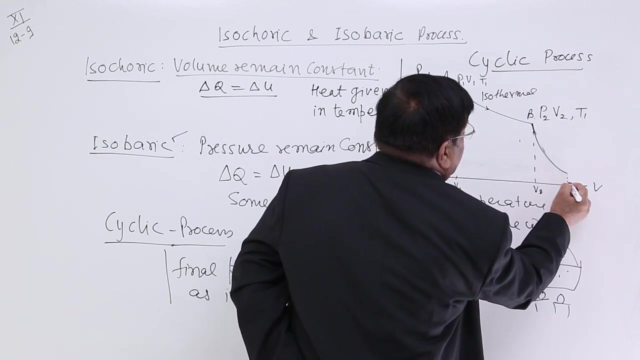 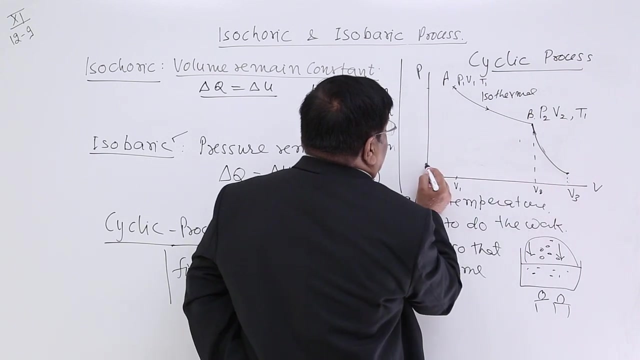 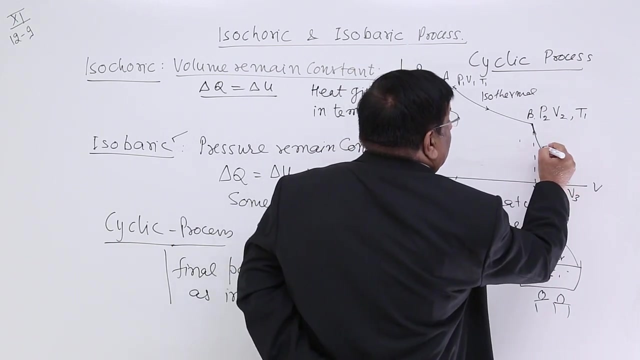 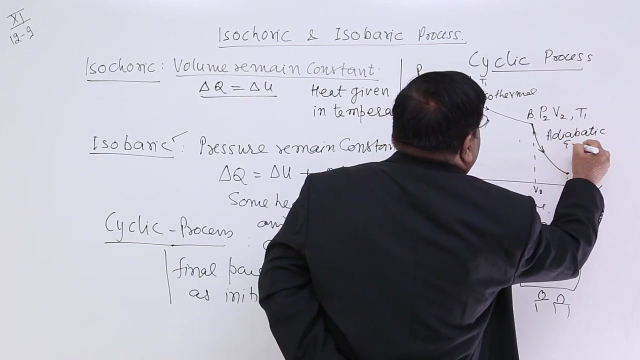 But now it decreases very sharply. So I get a graph here like this: So here is expansion done from V2 to V3 and the pressure has decreased to this level is P3.. This level was P2.. So this is again expansion. What is this? Adiabatic expansion, and we have reached P3V3.. Because 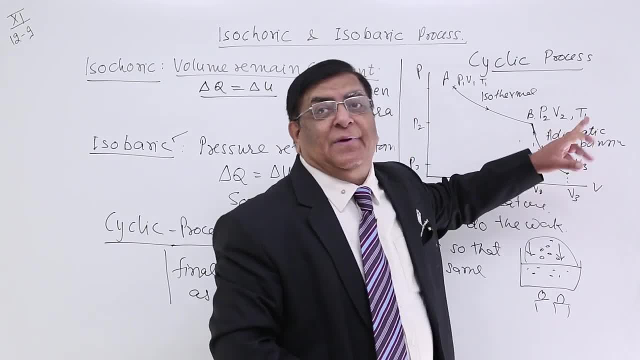 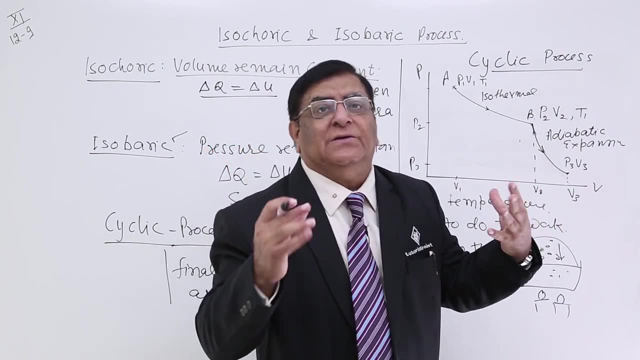 this is expansion. adiabatic in adiabatic, we do not allow heat to transfer. As a result, the temperature goes up or decreases. It is expansion: the temperature will come down. Whatever is the new temperature. we call it T2V3.. Now we write the temperature changing. 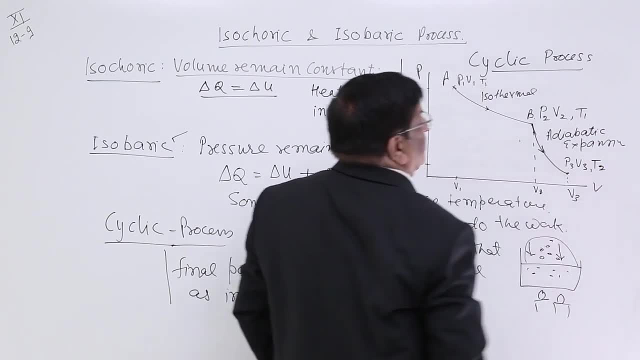 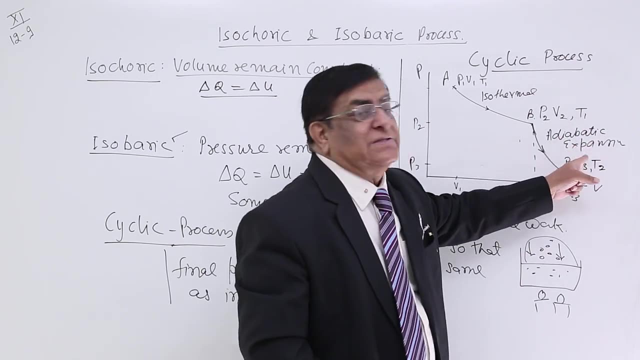 We won't pay for this temperature transfer, So we have to keep adding new temperature, temperature T2.. So the temperature changes, pressure changes, volume changes, temperature changes because it is adiabatic and the heat remain inside. Now, at this we have expanded. 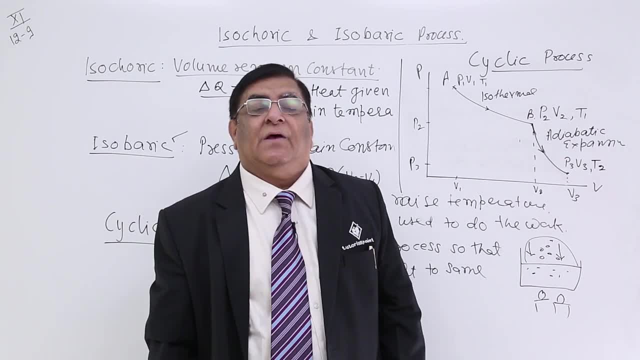 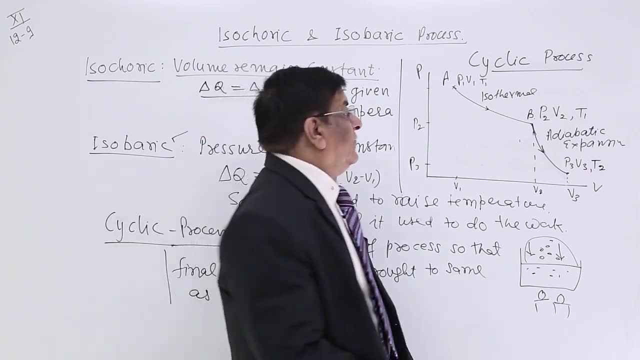 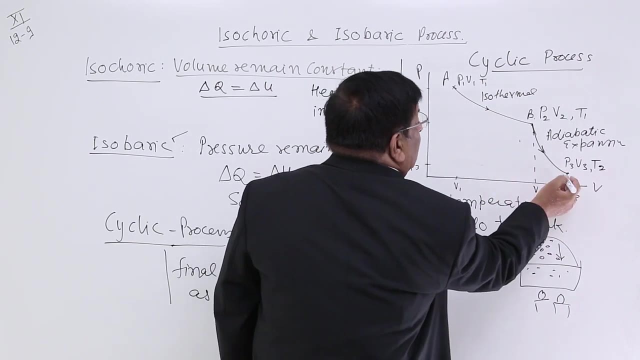 it by both the process. Now we compress it First, we compress it by slow method, that is isothermal method. So in isothermal method we keep on compressing, The volume become less, the pressure become more and our graph goes like this: The volume has become less. 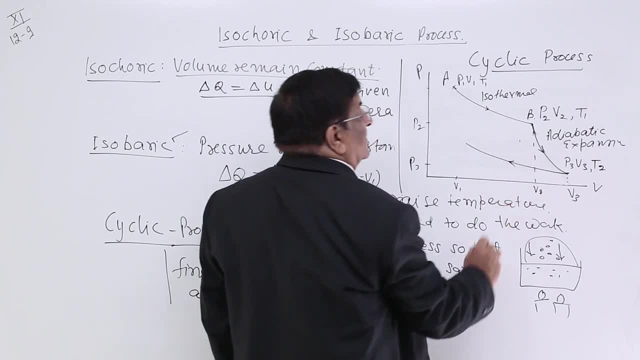 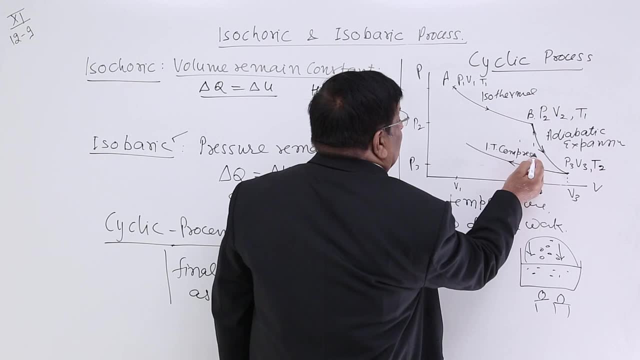 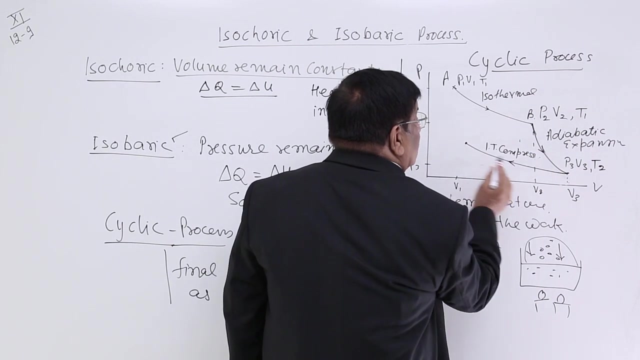 the pressure has become more and this is the direction of process. and what is this? Iso thermal compression In isothermal. what happens to temperature? The temperature do not change. therefore, the pressure and volume has changed to the value P4, V4, but temperature has not. 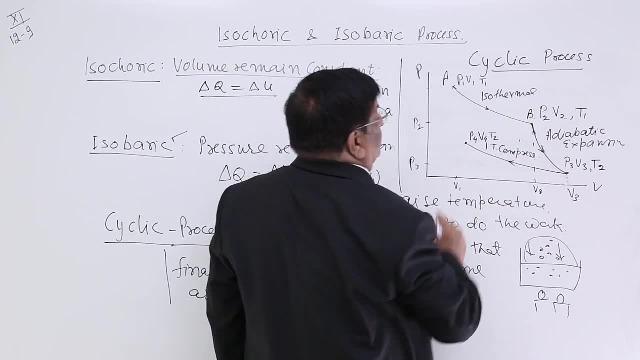 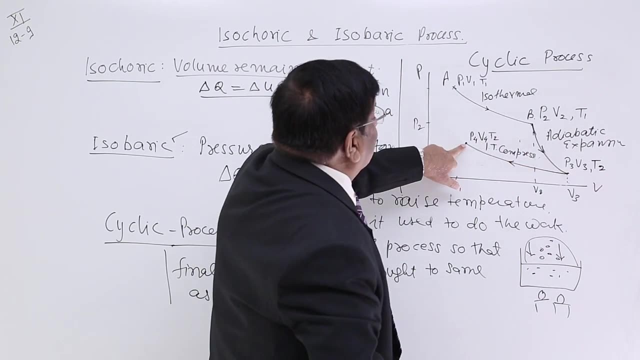 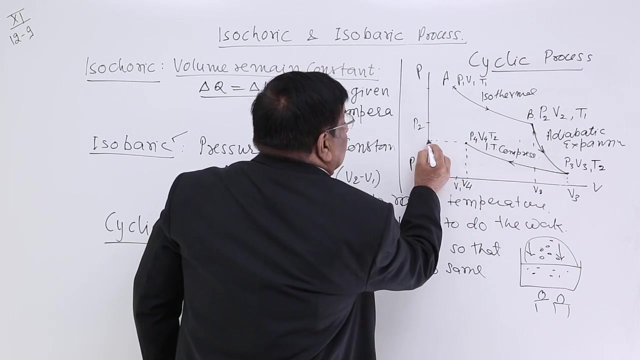 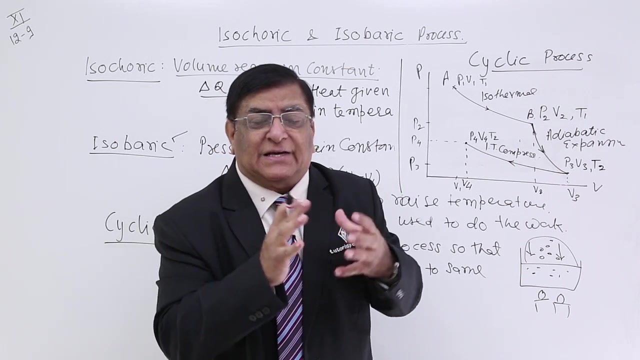 changed. it remain T2.. So this is the third process. first, second, third. Now, at this point, at this particular volume, V4 and this pressure, P4.. After this, we compress the gas suddenly. When we compress the gas suddenly in a quick, 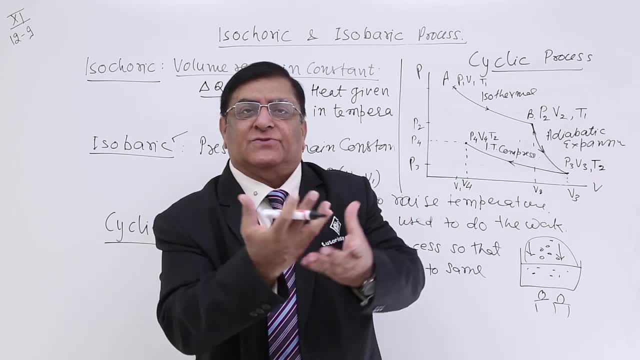 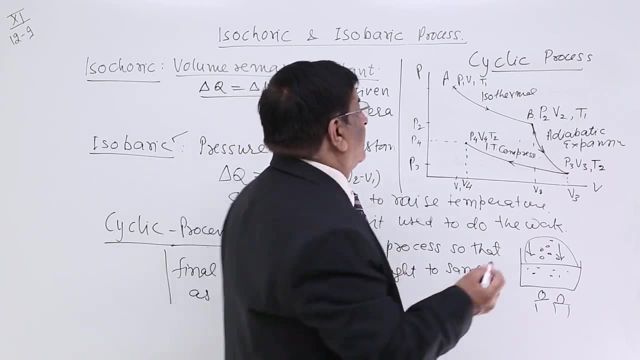 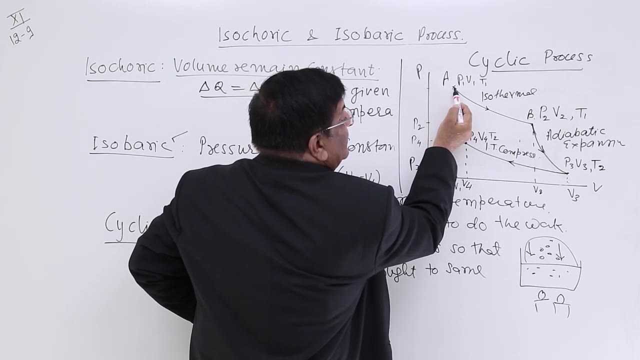 manner. the temperature goes high and we keep it in ensulated pot and that is adiabatic compression. In adiabatic compression, volume will become less, pressure will become high and temperature, which had become less. now we have to become high and we go from T2 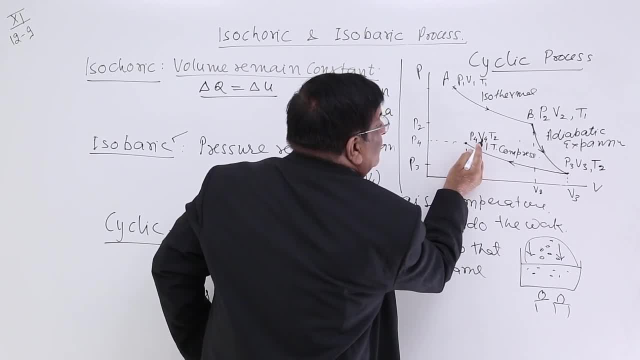 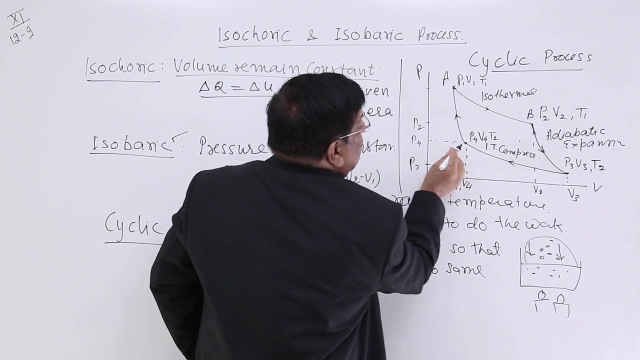 to T3. Making the pressure come, make it in to T2, shoot way and above it, helps the temperature, compress it to the volume V1. With that the pressure become P1 and the temperature rise to T1. We reach the same point and here is the direction of process compression. What 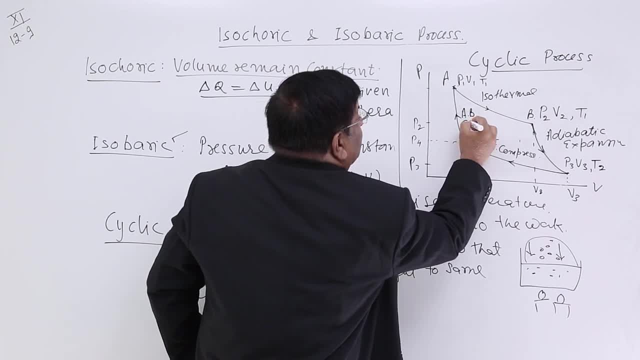 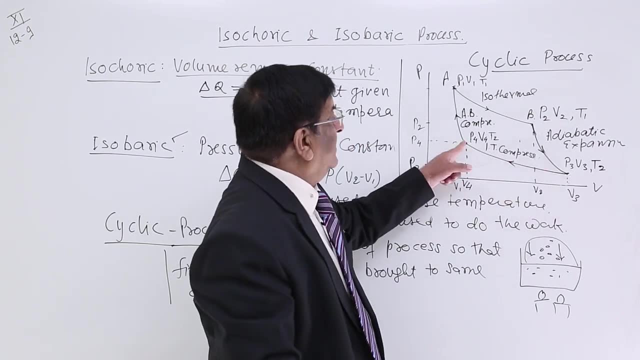 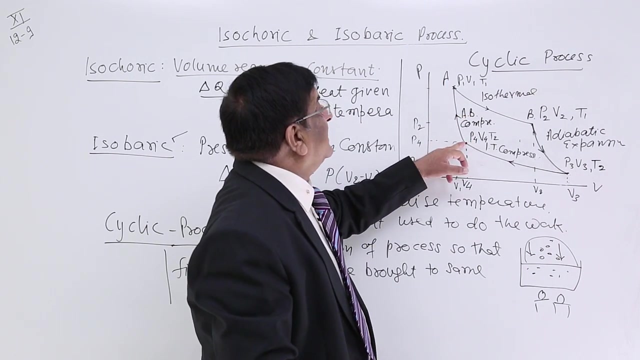 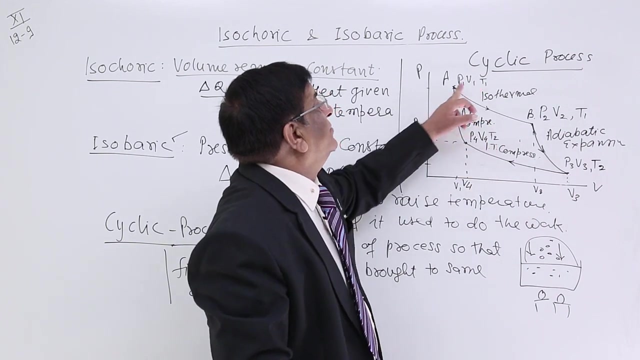 type of compression. it is Adiabatic compression. So this was isothermal compression. This is adiabatic compression and after this fourth process the pressure has increased to P1,, volume has decreased to V1 and temperature has increased to T1. The process is complete.